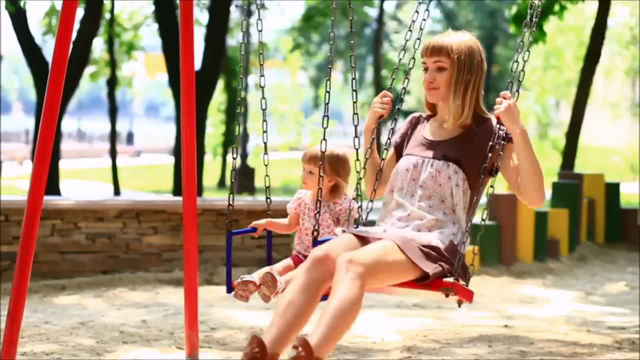 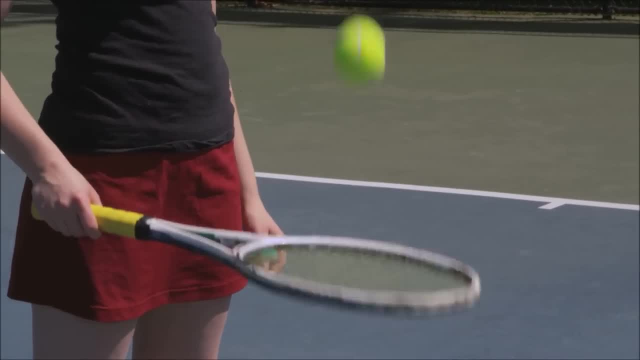 In order to start swinging you have to use a lot of force, but once you get going, it can be hard to stop. Here on Earth, there are some forces working on objects all the time. When you throw a ball upward, you can throw a ball backwards. When you throw a ball backwards, you can throw 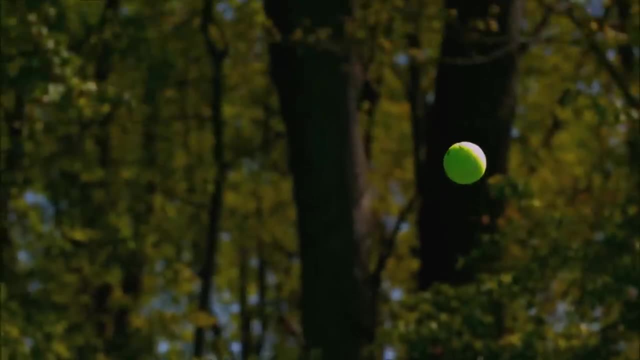 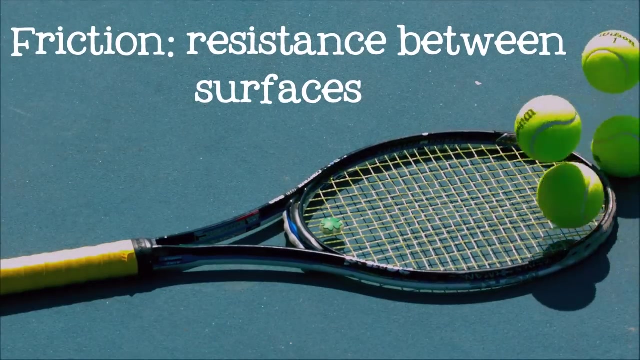 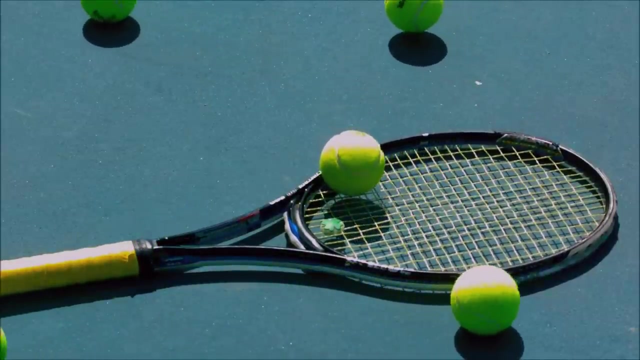 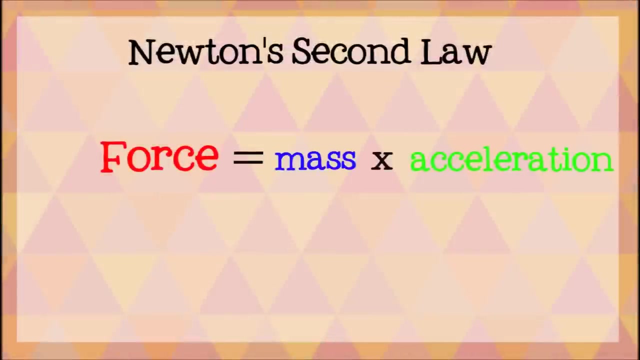 a ball in front of it. It doesn't keep going up forever, because the force of gravity pulls it downward. Once it hits the ground, friction — or resistance caused by surfaces rubbing together — will eventually bring it to a stop. Newton's second law says the force is the product of mass. times, acceleration: Mass is. 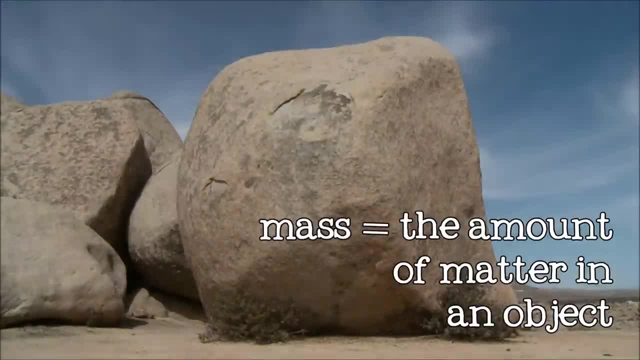 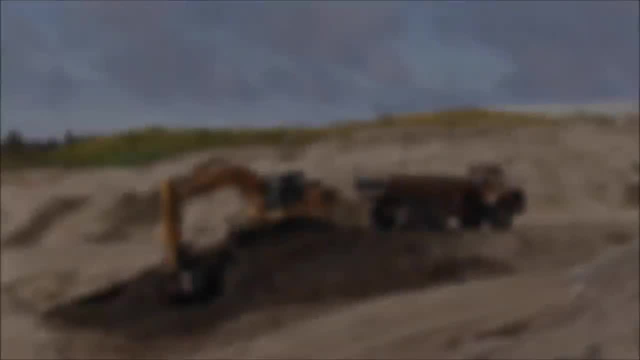 the amount of matter — or hair — which breaks by giving it a certain range, which is called mass. The mass of that mass is unique. by topicег stuff in an object To make something accelerate or speed up, you have to apply a force: The 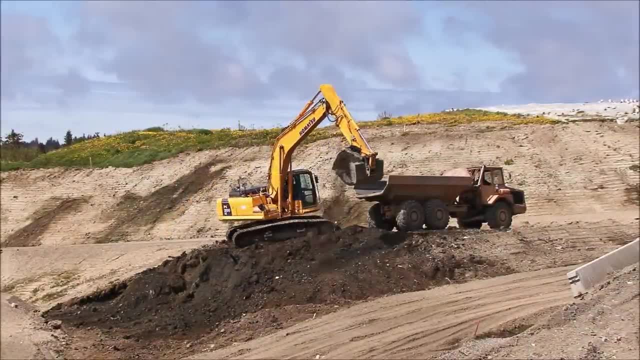 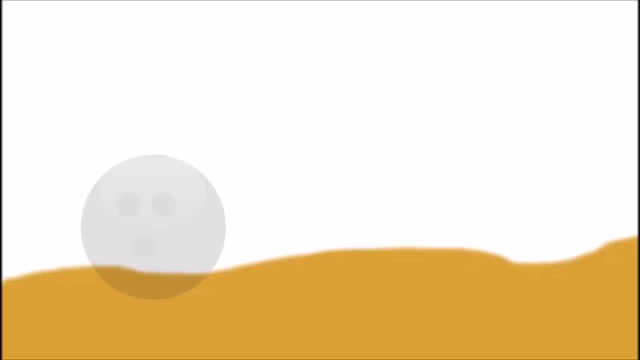 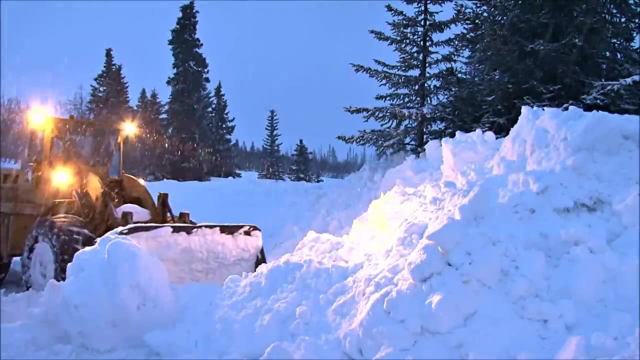 amount of force it takes to move an object changes depending on how massive it is. Think about it: You would need more force to move a bowling ball than to move a beach ball of the same size. The greater the mass of the object, the more force it will take to accelerate. 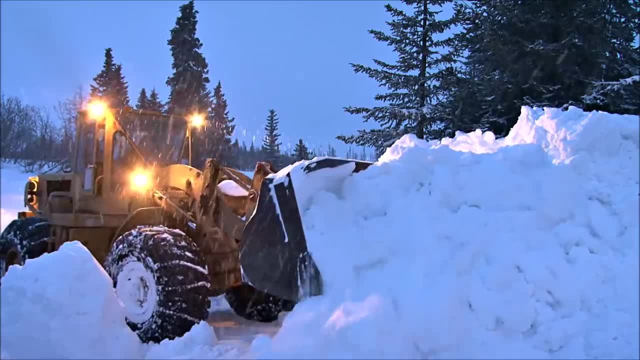 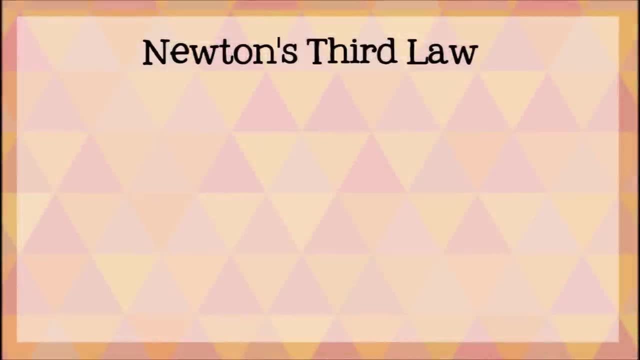 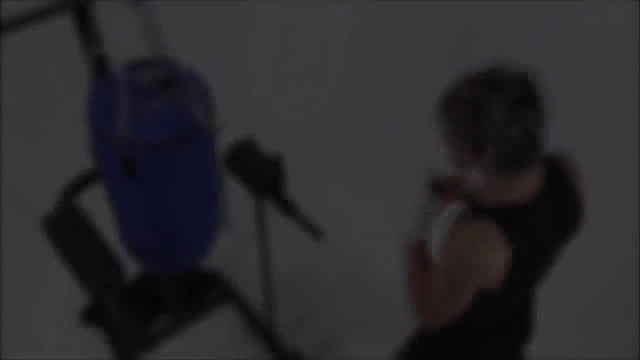 the object, and applying more force will make the object move faster. Newton's third law of motion says that for every action there is an equal and opposite reaction. If you exert a force on an object, it exerts an equal force back on you. 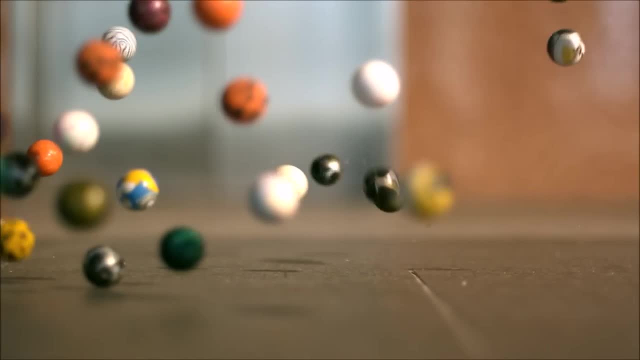 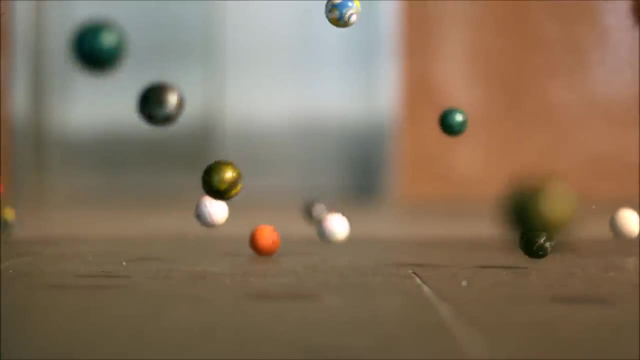 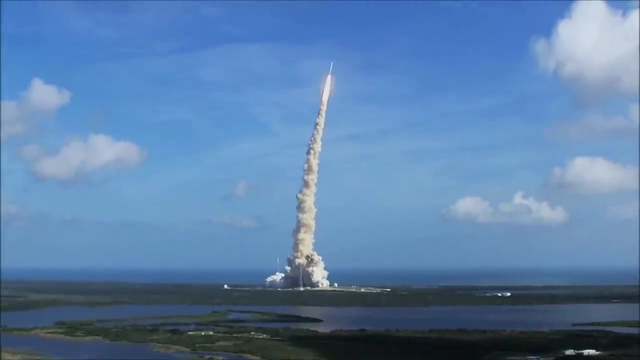 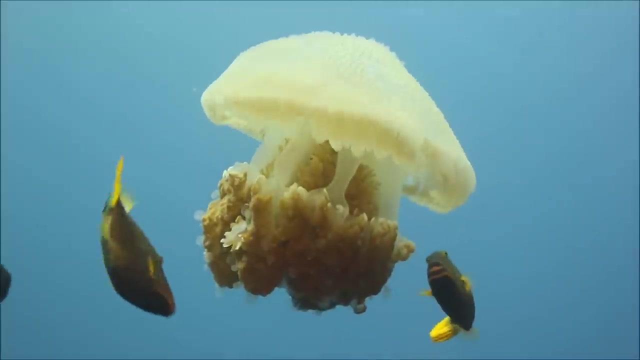 For example, a ball hitting the ground exerts force downward, The floor exerts an equal force upward. This is the principle that allows rockets to launch or jellyfish to swim: By exerting a force downward, an equal and opposite force pushes upward and the object accelerates.